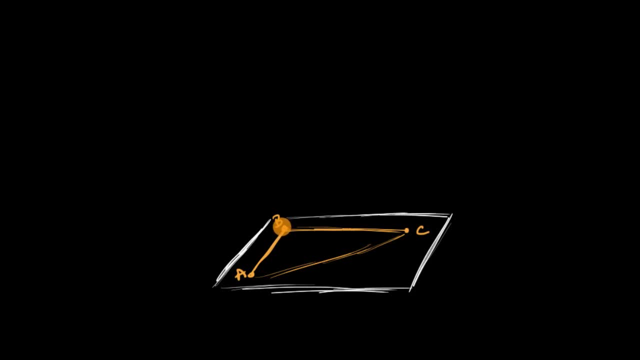 that's not on the surface of this desk and it's going to be right above point B, So let me just take that point, go straight up and I'm going to get to point P right over here. Now what I can do is construct a pyramid. 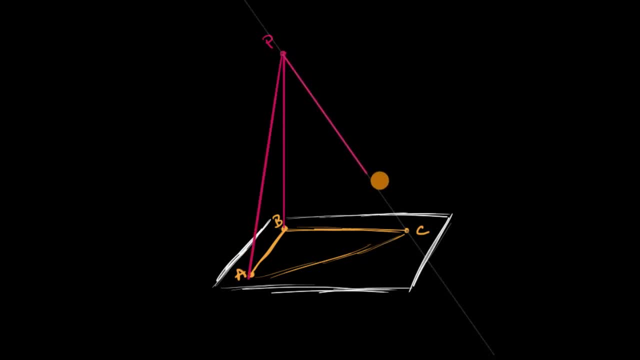 using point P as the peak of that pyramid. Now, what we're going to start thinking about is what happens if I take cross sections of this pyramid. So in this case, the length of segment P B is the height of this pyramid. Now, if we were to go halfway along that height? 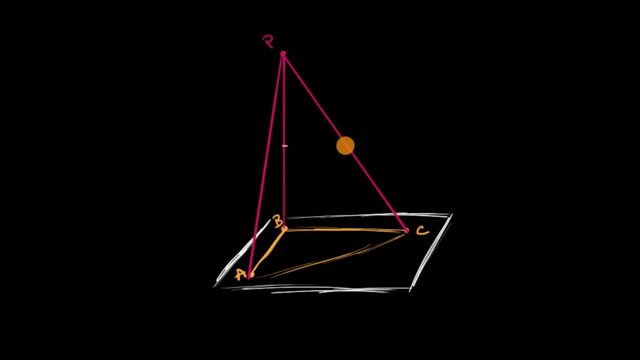 and if we were to take a cross section of this pyramid that is parallel to the surface of our original desk, what would that look like? Well, it would look something. it would look something like this: Now you might be noticing something really interesting. 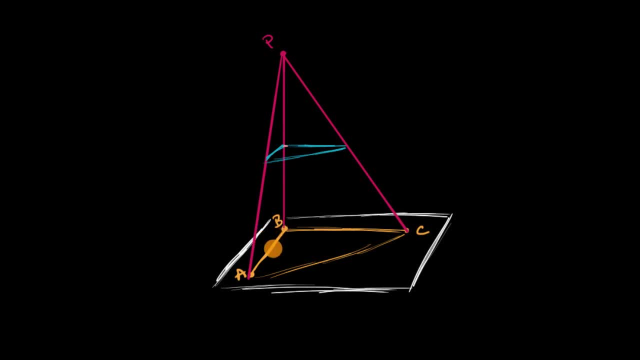 If you were to translate that blue triangle straight down onto the surface of the table, it would look like this. And when you see it that way, it looks like it is a dilation of our original triangle centered at point B. And in fact it is a dilation centered at point B. 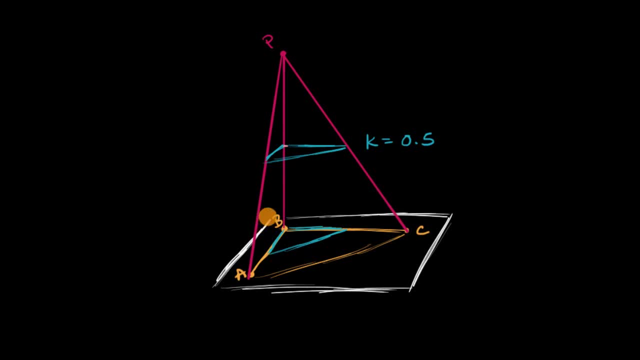 with a scale factor of 0.5. And you can see it right over here. This length right over here, what BC was dilated down to, is half the length of the original BC. This is half the length of the original AB. 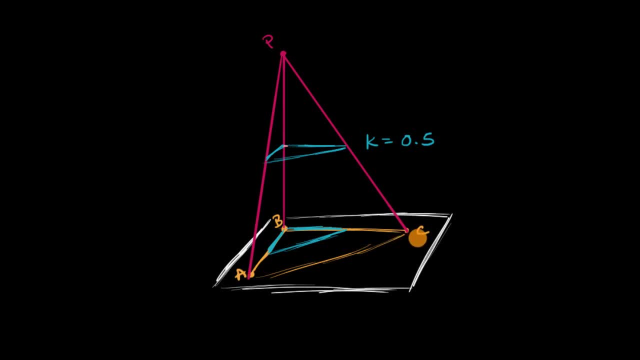 And then this is half the length of the original AC, But you could do it at other heights along this pyramid. What if we were to go 0.75 of the way between P and B, So if we were to go right over here? 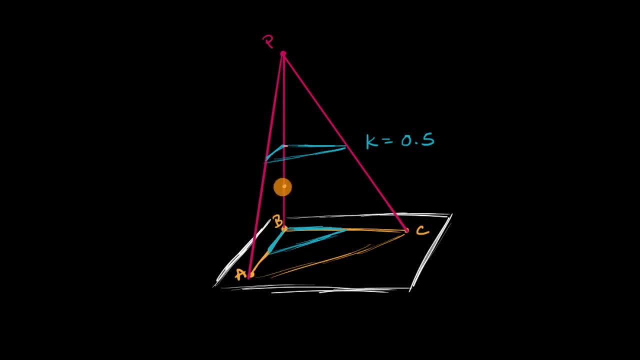 So it's closer to our original triangle, closer to our surface. So then the cross section would look like this: Now, if we were to translate that down onto our original surface, what would that look like? Well, it would look like this: 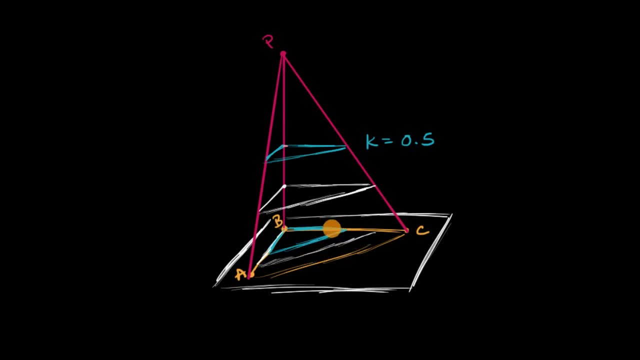 It would look like a dilation of our original triangle centered at point B, but this time with a scale factor of 0.75.. And then what if you were to go only a quarter of the way between point P and point B? Well then, you would see something like this: 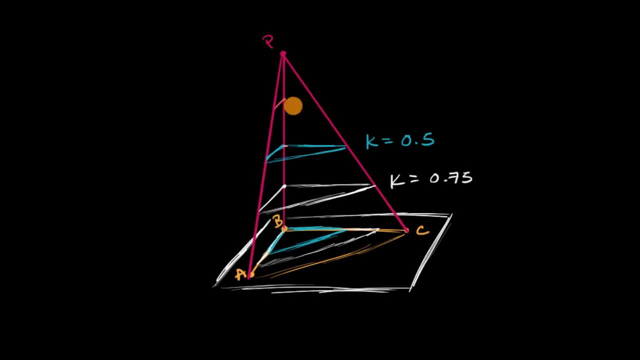 A quarter of the way. if you were to take the cross section parallel to our original surface, it would look like this: If you were to translate that straight down onto our table, it would look something like this: And it looks like a dilation centered at point B. 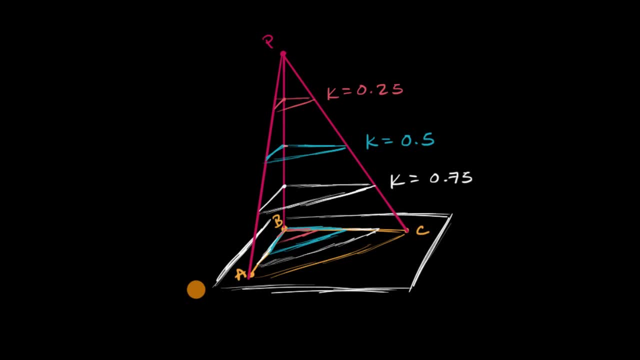 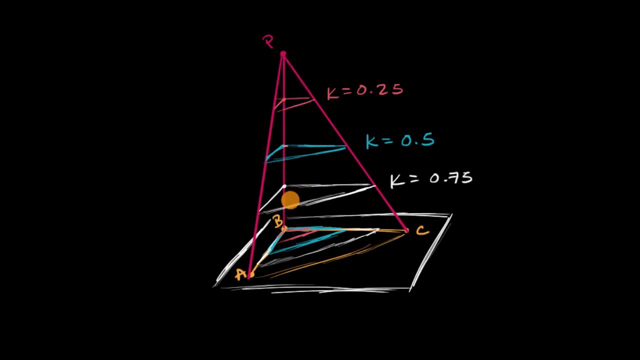 But this is a way to conceptualize dilations, or see the relationship between cross sections of a three-dimensional shape, in this case like a pyramid, and how those cross sections relate to the base of the pyramid. Now let me ask you an interesting question. 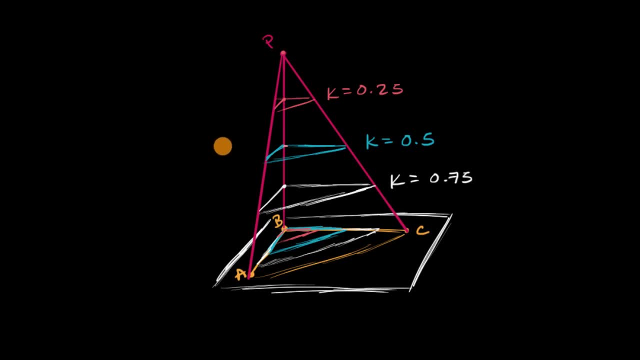 What if I were to try to take a cross section right at point P? Well then I would just get a point. I would not get an actual triangle, but you could view that as a dilation with a scale factor of 0.. And what if I were to take a cross section at the base? 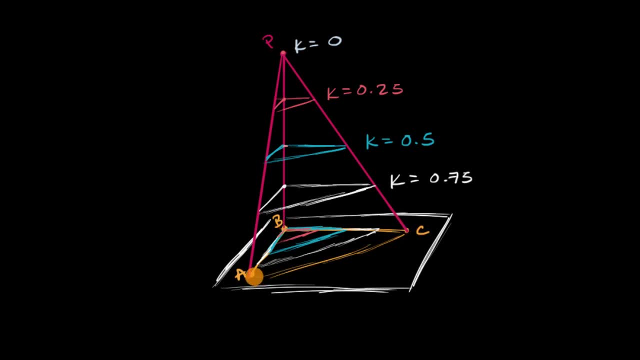 Well then, that would be my original triangle, triangle ABC, And then you could view that as a dilation with a scale factor of 1, because you've gone all the way down to the base. So hopefully this connects some dots for you between cross sections of a three-dimensional shape. 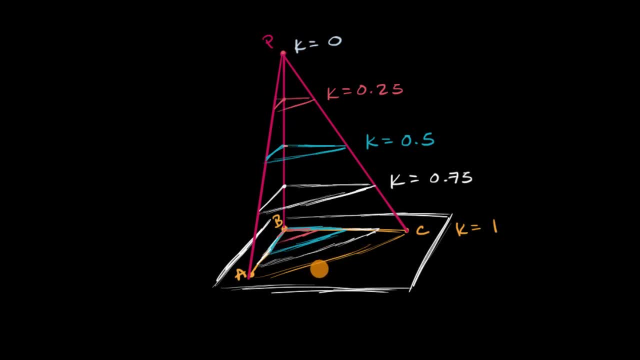 that is parallel to the base and notions of dilation.